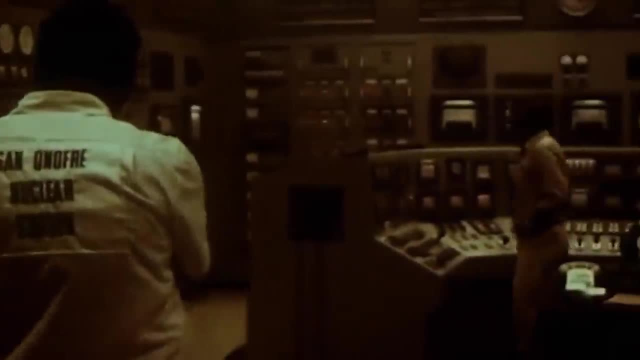 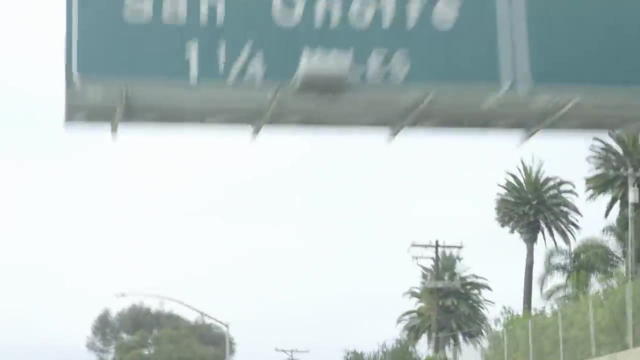 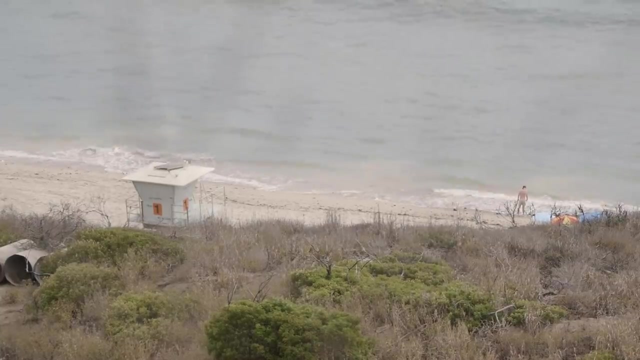 Back when it was running, the San Onofre plant could power 1.4 million homes at a time. But now the reactors are retired and the plant's operator, Southern California Edison, is preparing to dismantle it completely. So to see this whole multi-billion dollar process firsthand, we took a tour of the power. 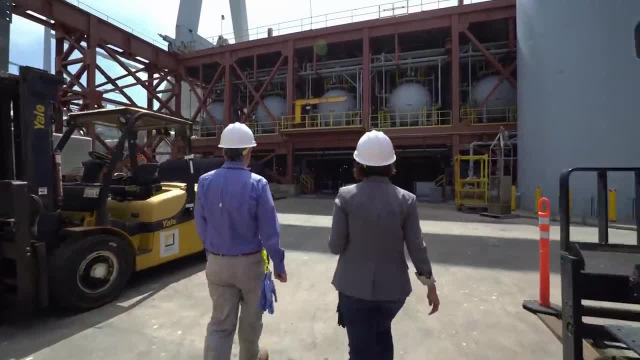 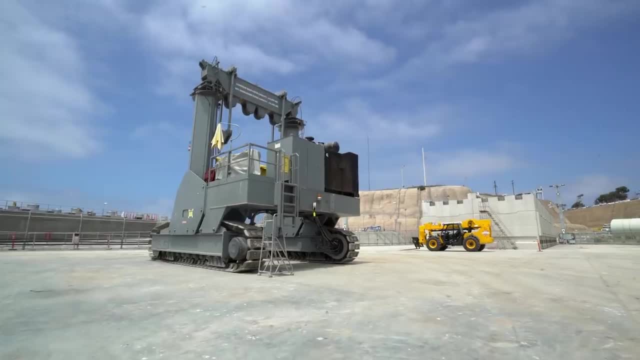 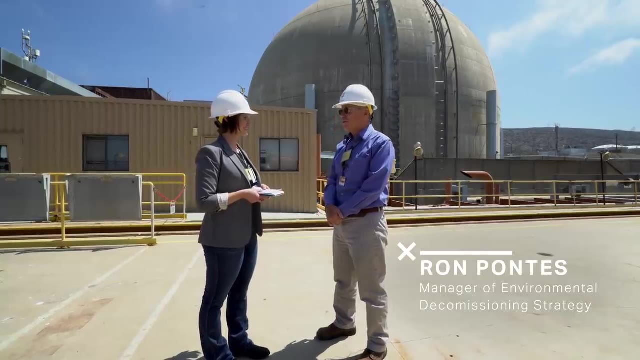 plant. Our guide is Ron Pontes, Manager of Environmental Decommissioning Strategy, And except for all of the security, the seagulls and us, the place is pretty empty. Behind us is the containment building for Unit 3.. Inside that building is the nuclear steam supply system, which consists of the reactor. 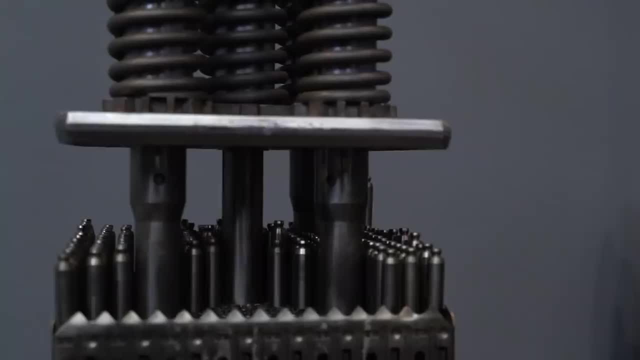 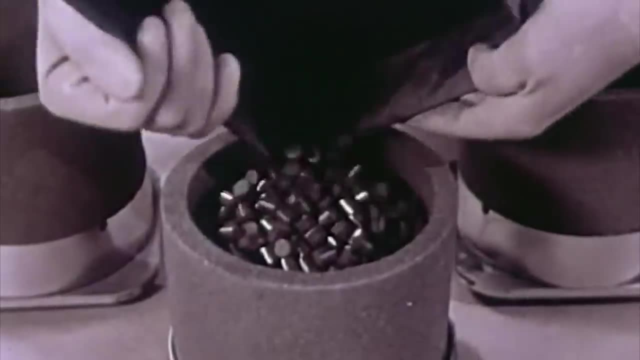 steam generators, pressurizer and reactor coolant pumps. That's where the fuel would normally go. Bundles of hollow metal rods that are packed with little pellets of uranium. Inside the reactor, uranium atoms split apart And that's where the fuel would normally go. 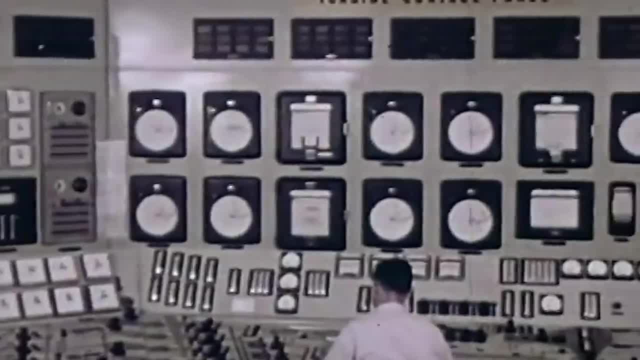 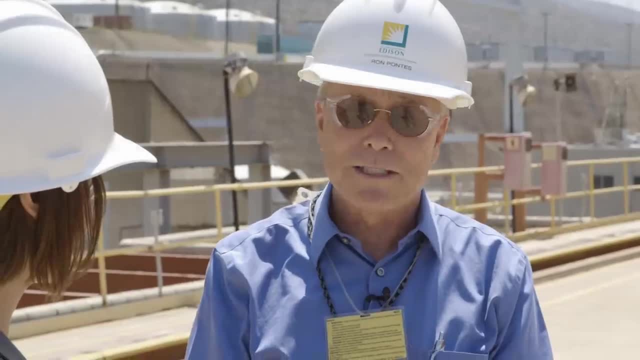 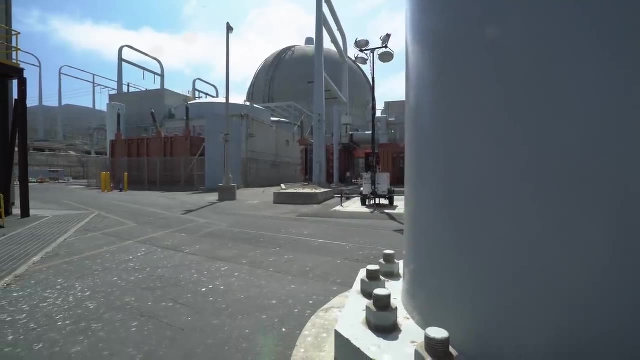 That's where the heat is generated. that is transmitted to the steam generators to make steam, to turn the turbines, which makes electricity for our customers. Only this plant hasn't produced electricity for years, ever since one of the steam generators sprung a leak. 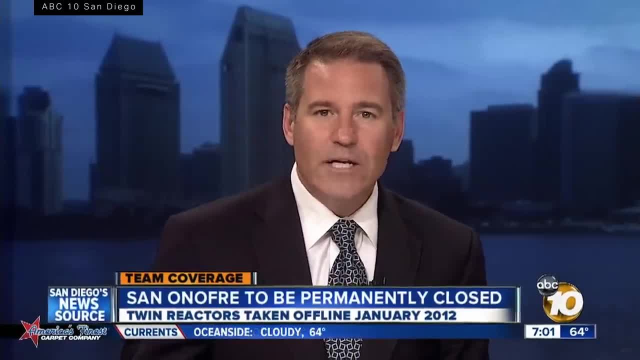 It is a done deal. SoCal Edison has gotten tired of waiting to reopen the troubled San Onofre power plant, so today the utility announced it is shutting it down for good. Now the plant operators need to get back to work. 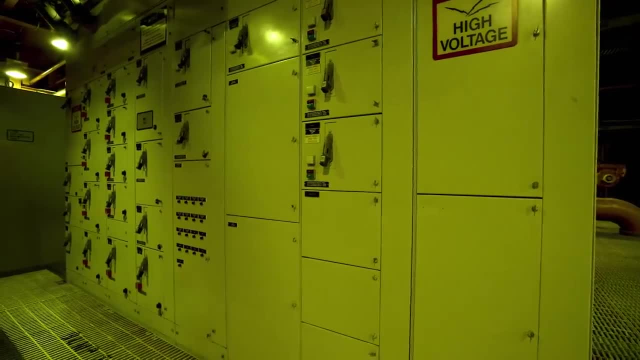 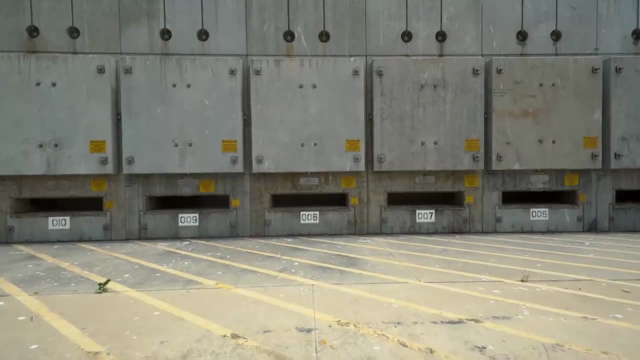 SoCal Edison has gotten tired of waiting to reopen the troubled San Onofre power plant. so today the utility announced it is shutting it down for good. First they have to do something with all of that fuel, Then they have to don something with all of the fuel. 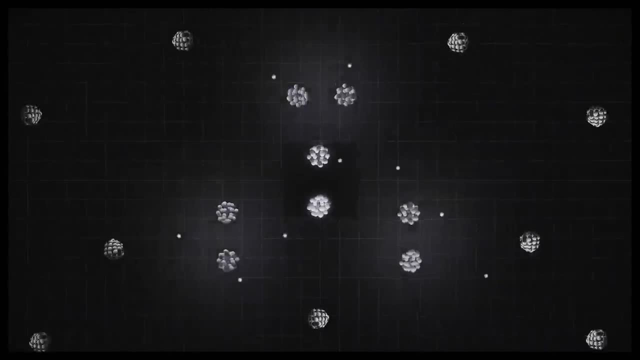 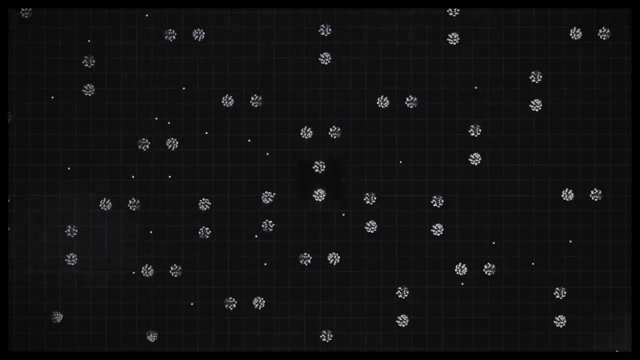 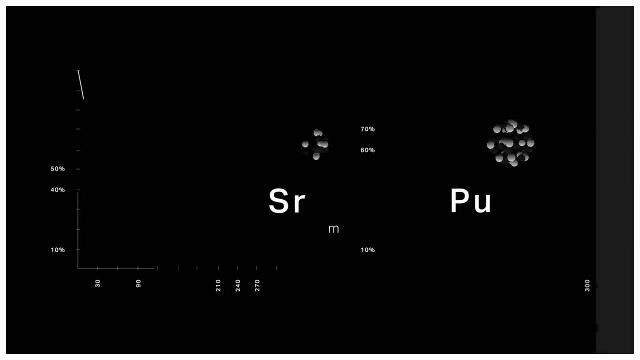 Fresh fuel isn't all THAT radioactive. It gets more dash new radioactive in a nuclear reactor, But without fresh uranium it gets really real chain reaction that generates heat. it also makes other radioactive atoms like cesium-137, strontium-90, and plutonium-239.. About half of the cesium and strontium decay in 30 or so years. 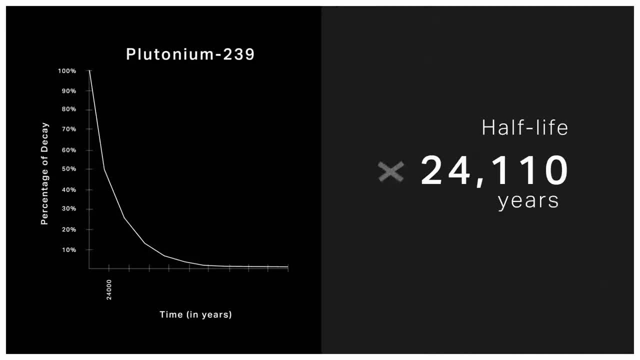 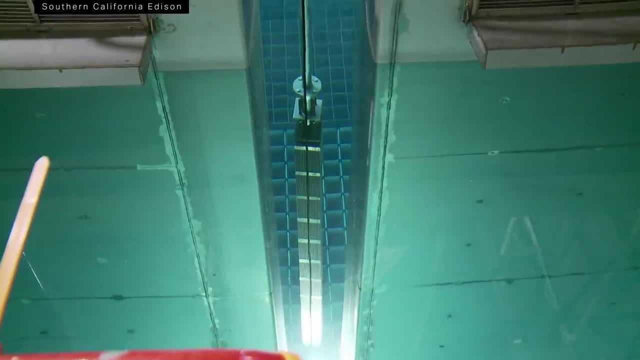 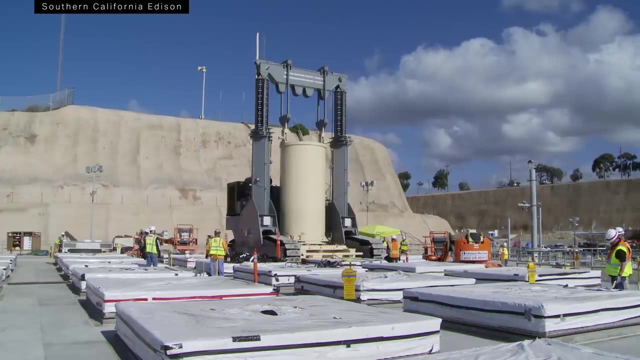 The plutonium That takes longer- Like 24,000 years longer. These days the spent fuel starts cooling off in cement-lined pools of water. After a few years it's moved to dry storage, Air-cooled steel containers inside massive concrete blocks. Eventually they'll move all. 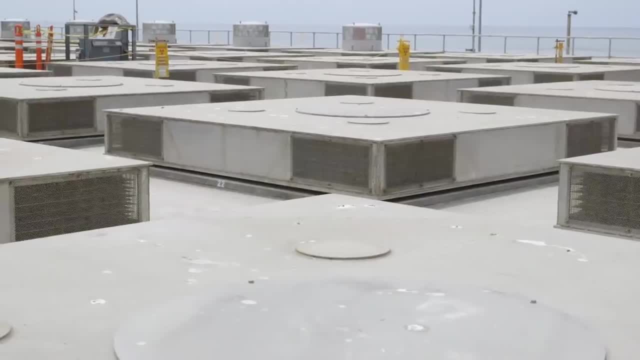 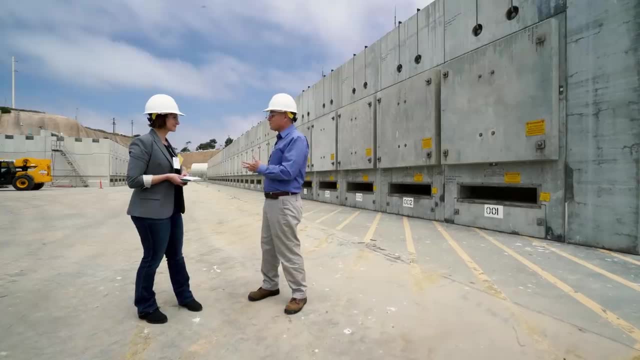 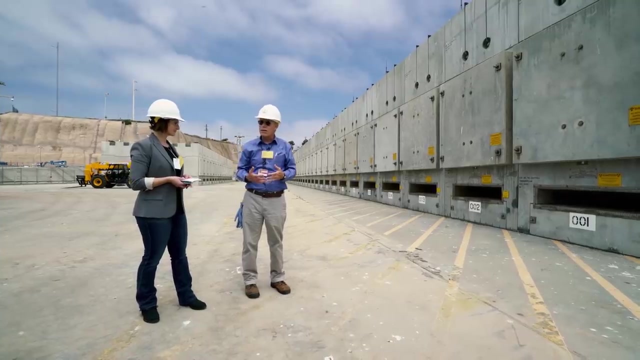 the waste into those blocks. They're lower maintenance and they're supposed to withstand floods, earthquakes, tornadoes, airplane collisions, you name it. It requires no pumps or active systems to support it, As long as we keep this inlet and outlet free of any debris or blockage. 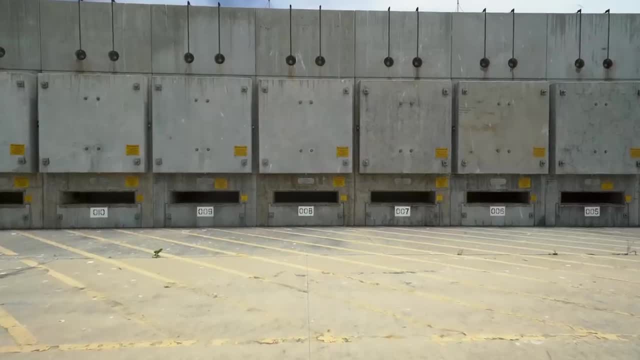 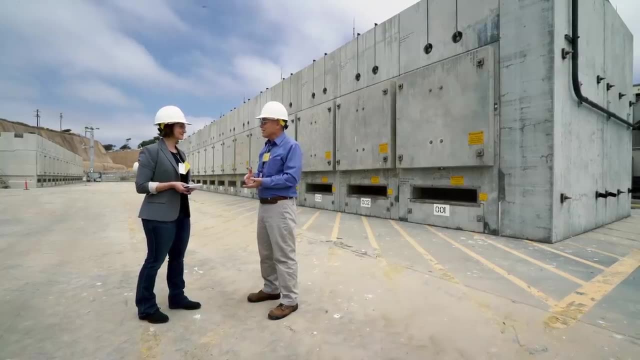 this system will continue to operate. That's good, because that's where the spent fuel is going to have to stay for the foreseeable future. What we are faced with here is a national problem. Every commercial plant in the states is faced with the same problem. There's nothing to do with the fuel. because the federal government's not performing San Onofre's first reactor, powered up in 1968, at the height of nuclear energy's prime and the height of the energy industry, selling America on how safe and powerful it was. The heat output of one pound of uranium can equal the heat output of 70 tons of coal. 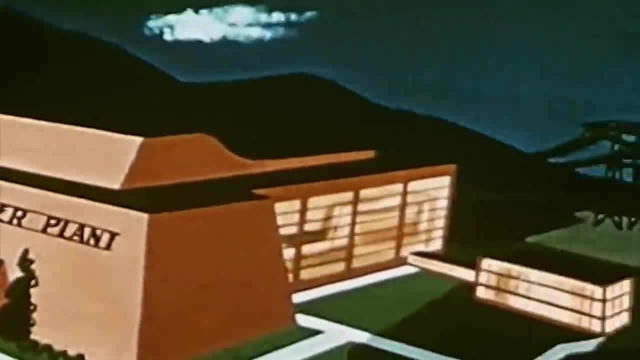 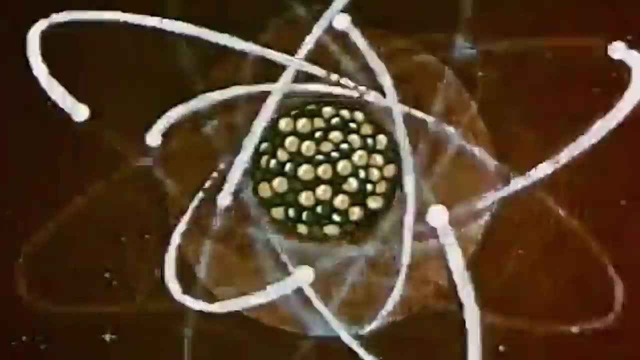 There were promises that one day atomizers would be able to produce more than one ton of coal, That atomic energy would be too cheap to meter, That it would power the world by the year 2000.. But for all that promise, there just wasn't a solid plan for the waste. 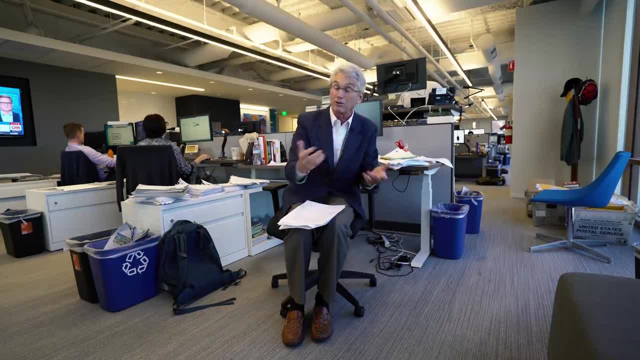 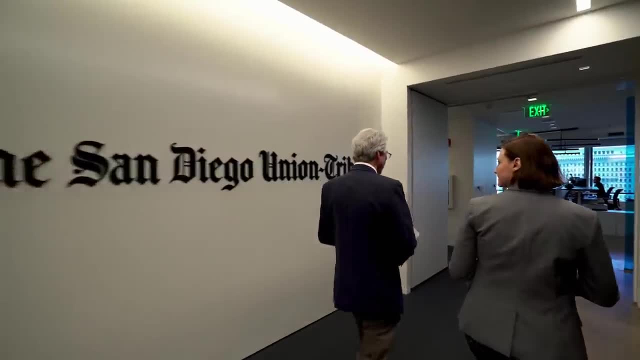 One could argue maybe we should have thought about this as a nation before we started building nuclear power plants. but by this time the horse is already out of the barn. That's Rob Nicoleski, a reporter at the San Diego Union-Tribune, who's been following. 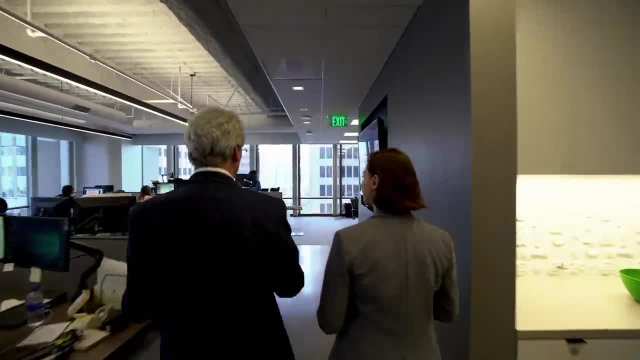 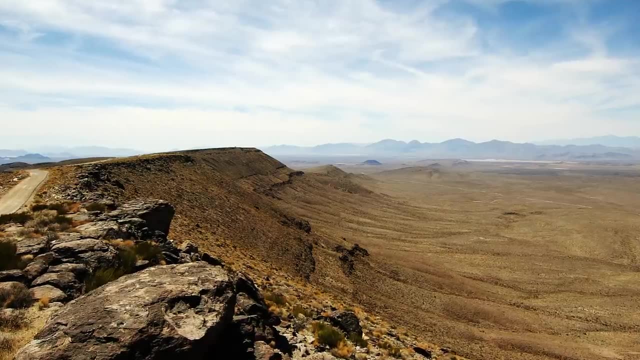 the story at San Onofre for years. In short, the reason why the spent nuclear fuel stays at San Onofre is because the federal government has dropped the ball. For decades the plan has been to bury the waste underground. The government was supposed. 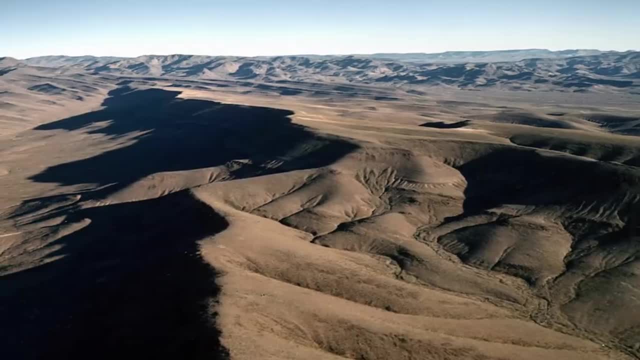 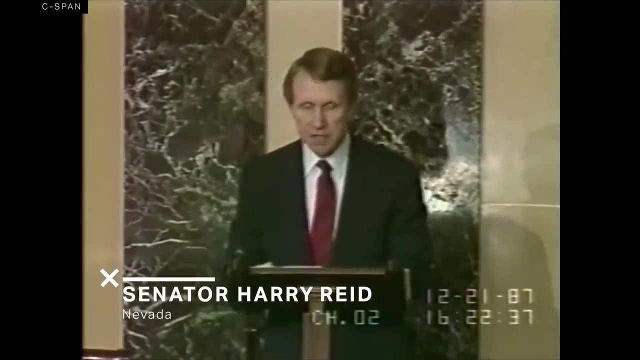 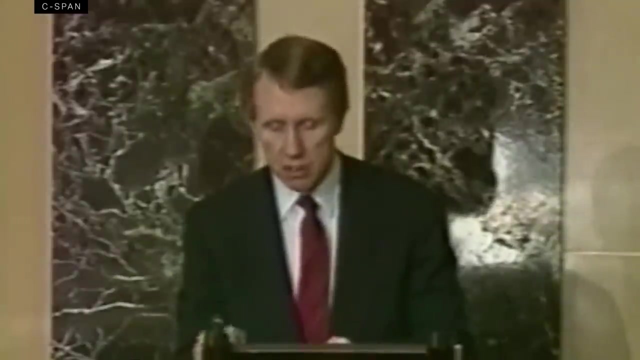 to start accepting spent fuel in 1998, and the site it settled on was Yucca Mountain in Nevada. Nevada politicians hated that idea. Beginning this year, the story takes a new and, yes, an ugly turn, which the press and others tagged months ago the Screw Nevada Bill. 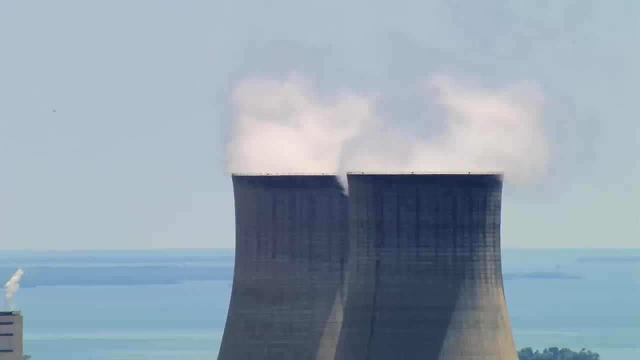 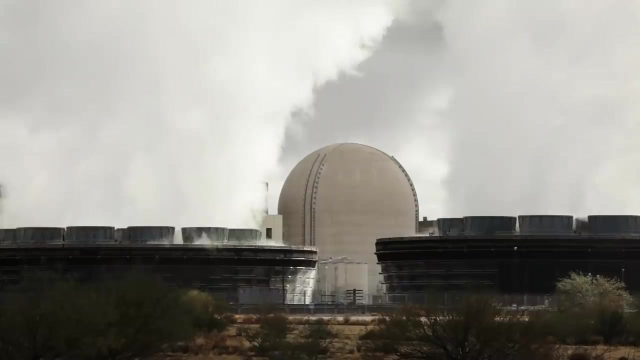 So the plan has been stuck in limbo for decades, and nuclear power companies have been suing the government for missing that deadline. Meanwhile, nuclear plants keep operating. They produce about 20 percent of America's electricity and 2200 tons of waste each year. 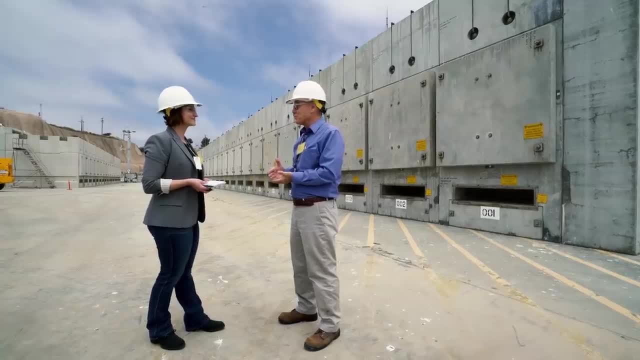 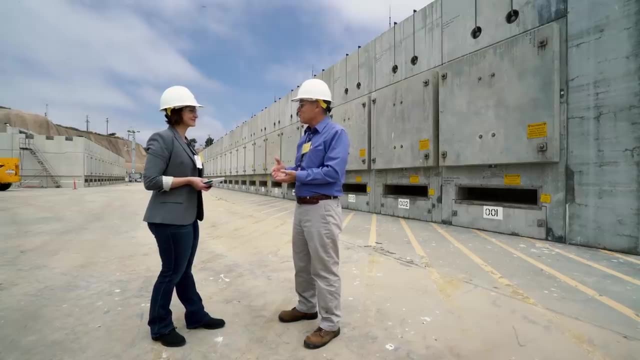 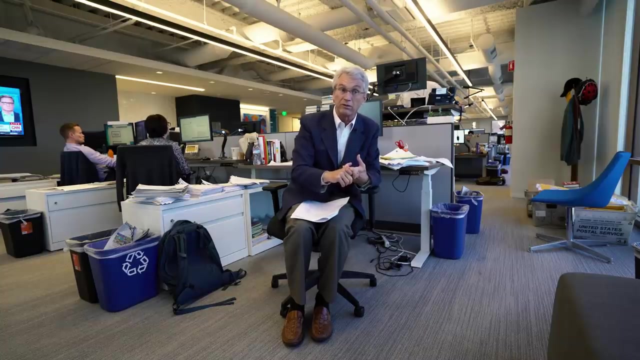 This is probably not the ideal place to store spent nuclear fuel- we would all agree on that- but while it's here, we will fulfill our obligation to manage it safely. There are a few ways out of this situation…. There's been a movement in Congress to restart Yucca Mountain. The Trump administration is